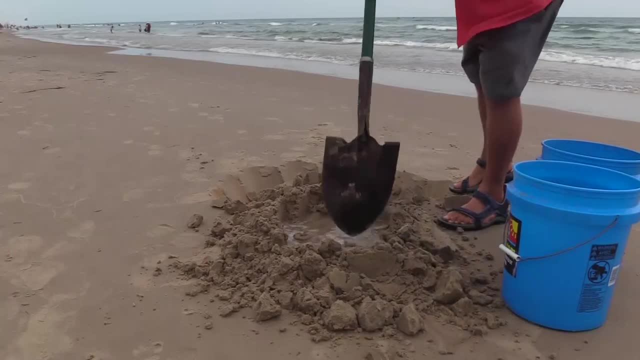 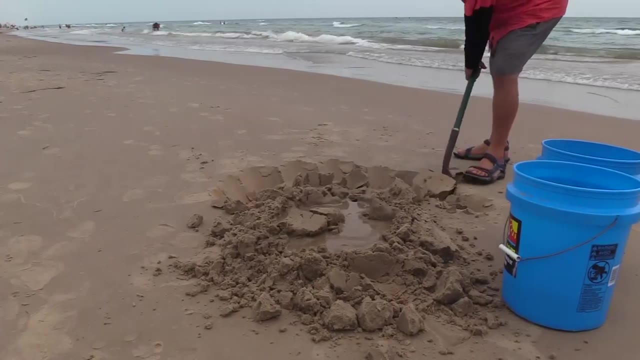 a little tower, a little volcano, and fill it full of water and put some sand in that- and we use science all the time in our lessons. so if our beach isn't quite level- which it isn't- we make a little volcano, so that gravity, once it's mixed with the sand and water and it's molten in the 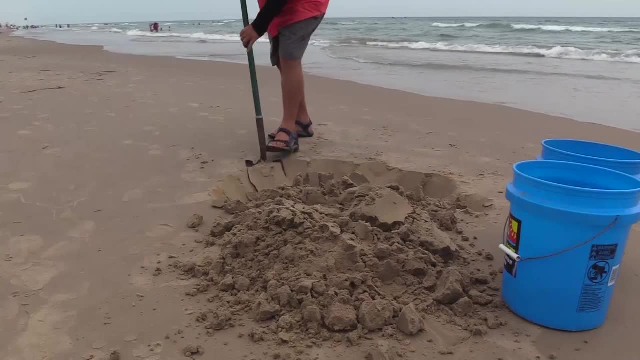 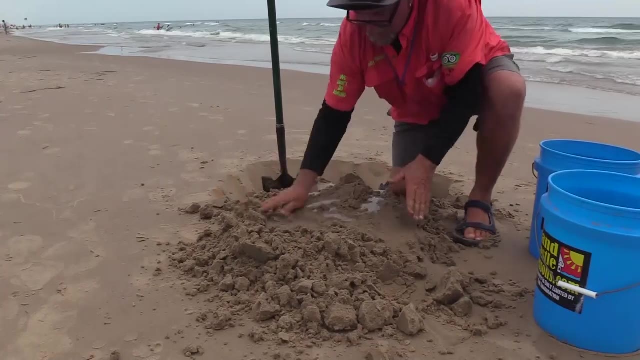 middle will level itself. so we know our little pad. when it's got water in the middle of it, we can spread the sand around with our hands, push it all up in the same place and we're going to get it virtually flat, which is what you want. you want your sandcastle sitting on a level base or an? 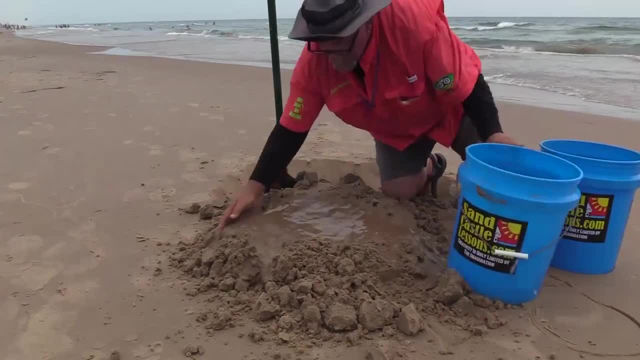 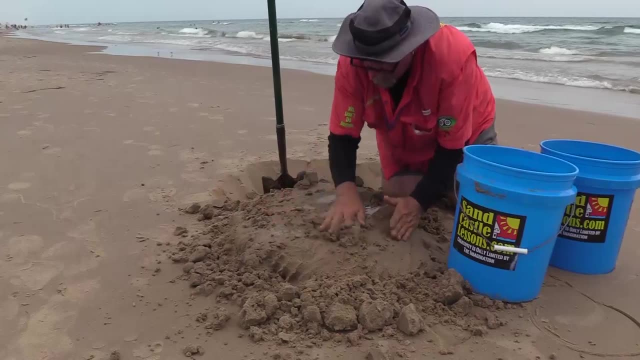 almost level base, because if you don't do that, gravity is going to be pulling on the side of so. what we do is we spread it out with our hands, make it a nice soft base. I mean, today's not about the base, but if you make a nice solid foundation like this, you won't have any problems with your 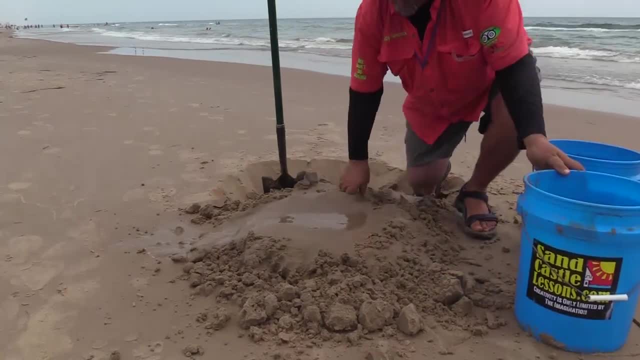 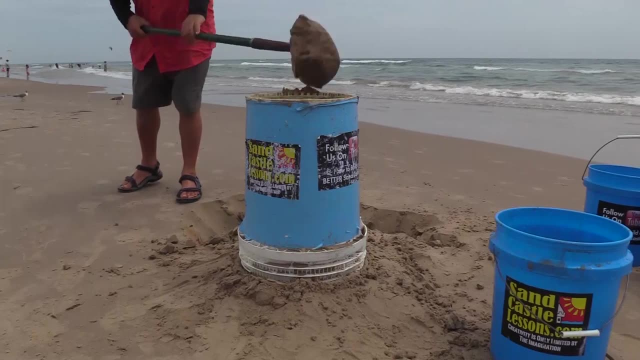 sandcastle falling over afterwards. we compact the sides with our feet and then we. then we get our big bucket- these are 100 pound chlorine powder buckets and which we wrap because they don't look very attractive, and you put the sand in them about a third of the way up and then you make a 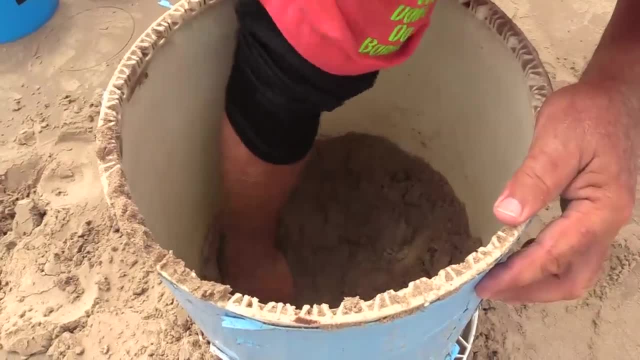 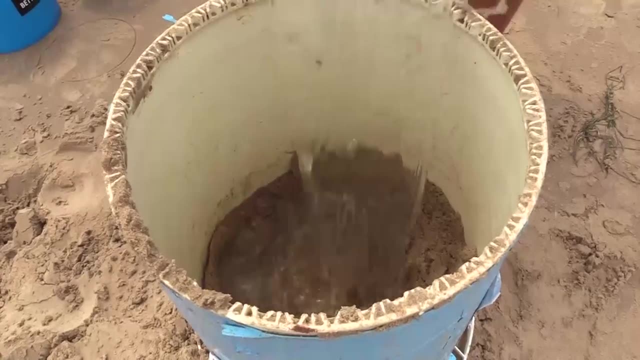 dish in the middle. you bash the middle down with your hand and then make a dish and then you pour the water into the center of that dish and then it won't blow the side of the bucket out. if you pour it down the side of the bucket, it just blows all the sand away and the water comes. 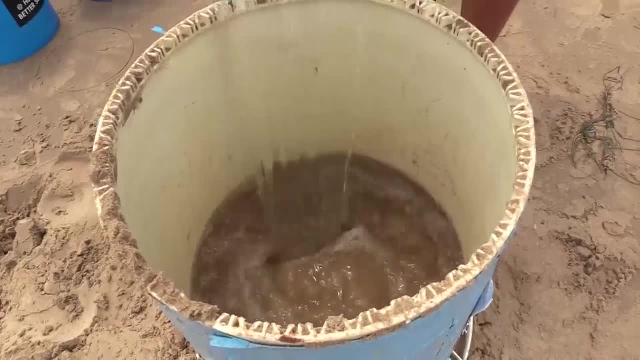 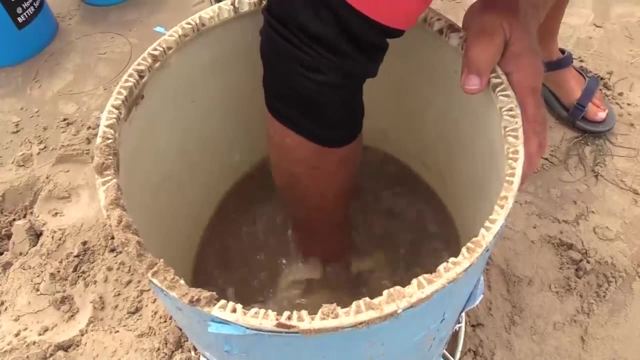 spewing out and away you go. so we put it in the middle of the bucket and that gives you what's called cavitation, and cavitation spreads the sand around the side of the bucket and it doesn't blow out. but we always give it a stir and make sure all that's thoroughly mixed, and then we put some. 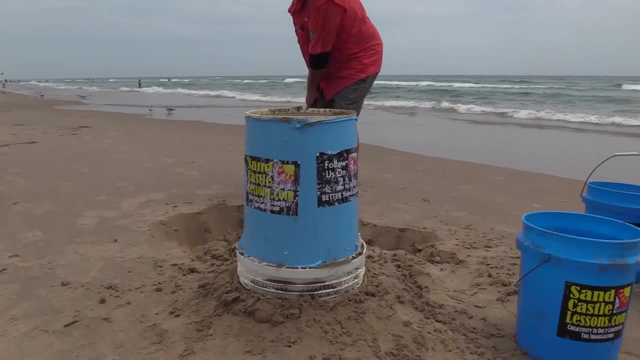 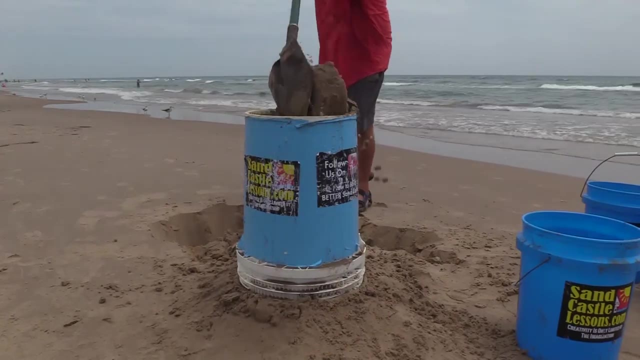 more water in the bucket and we add sand to water. now, the reason we add sand to water is because it does two things. number one: if you've got a bit of trash on the beach, uh, we haven't. we've got a lovely beach, um, but if you've got a bit of trash and seaweed and whatever. 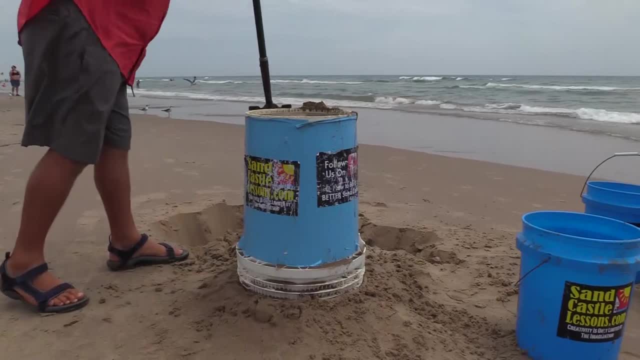 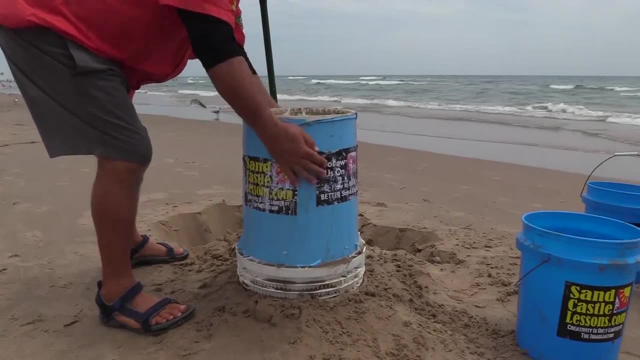 it'll lift that to the top and it'll float, obviously. and then when you compact it like this, we can wobble the bucket around. it's a bit of squidging and then a bit of tapping, and the tapping causes granulation and compaction and what that is is the smaller sand crystals float to the 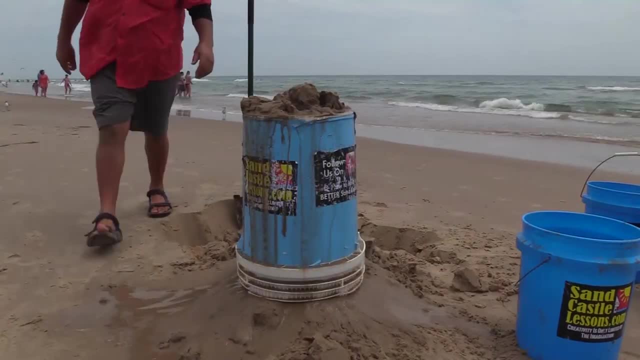 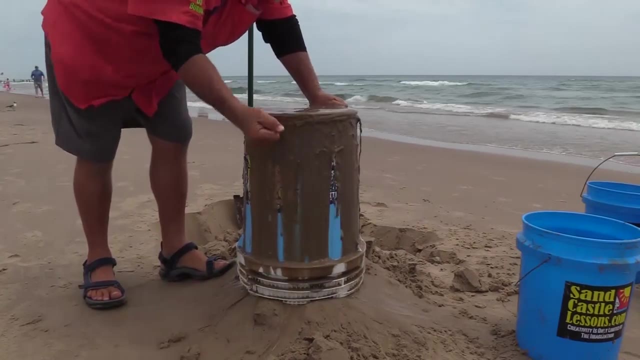 bottom and make this block very, very strong. the other thing it does is it takes all the air out of the. when you're tapping this, all the air is coming out between the sand crystals and the water powder, so all the stones. so there you go. so that's that's why we do this. we tap it and we use so much. 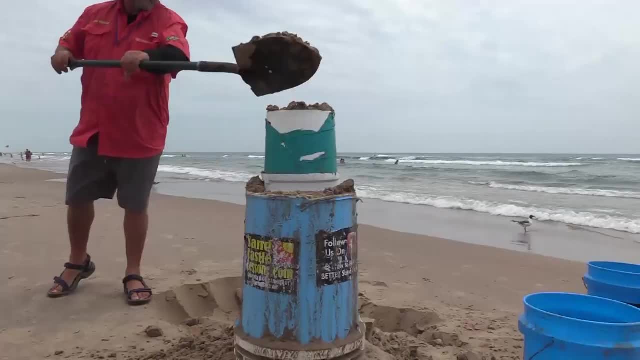 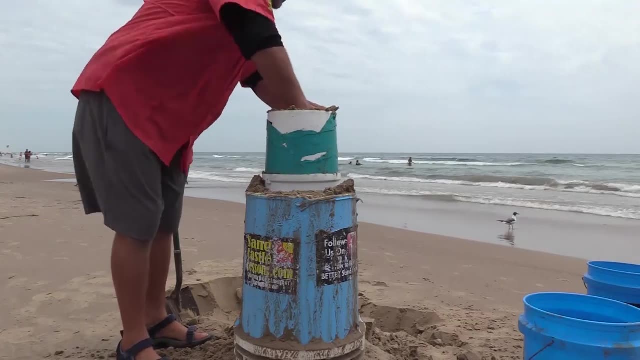 water and we add sand to water. it takes the air out and gets the trash away. and then we put the smaller bucket on about about a third full again. make the dish in the middle. you can see my hand bashing the dish in the middle. put a bit of water in. that means it's penetrating all the way to the. 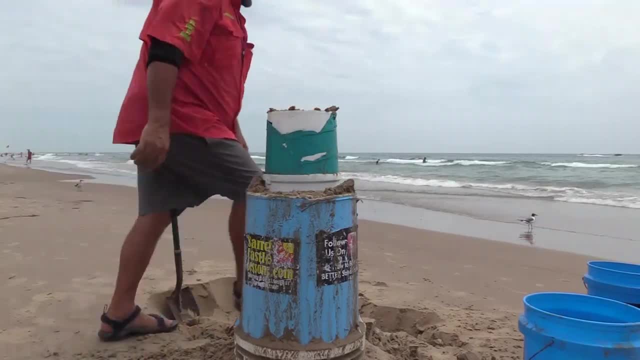 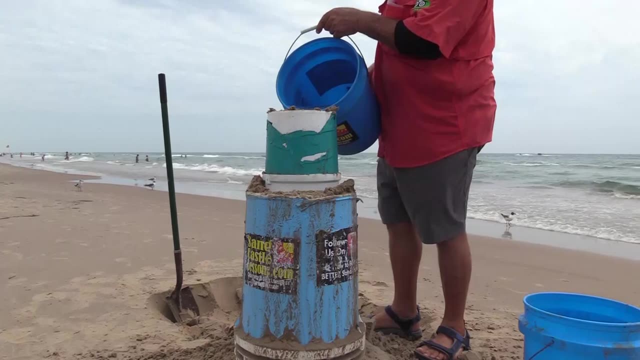 bottom and pop some water in there, and uh, water is vital. just if you're on a beach where, where you don't have sand to do this. uh, there are beaches where this doesn't work at all, because the crystals have got fractured surfaces or they're just not very flat, um, so it doesn't matter how. 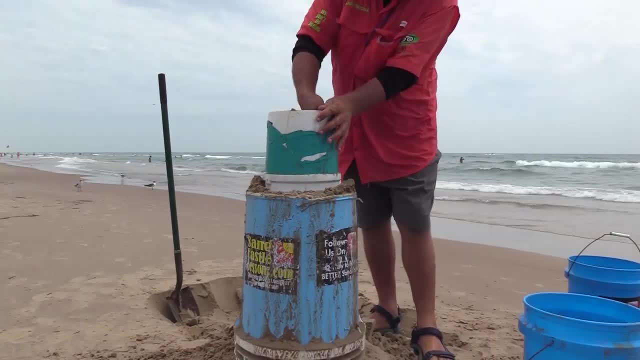 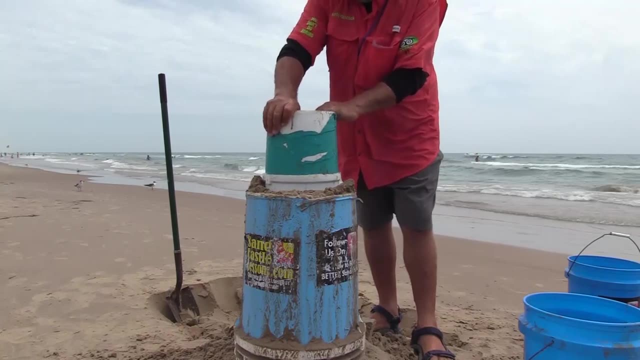 much water you put in there, they won't hold themselves together because they haven't got enough surface areas to do it. so that's why some sand works and some doesn't. we're very lucky, our sand is very sharp, which means flat, and it's very fine- about 400 grain so, which is very fine. so you 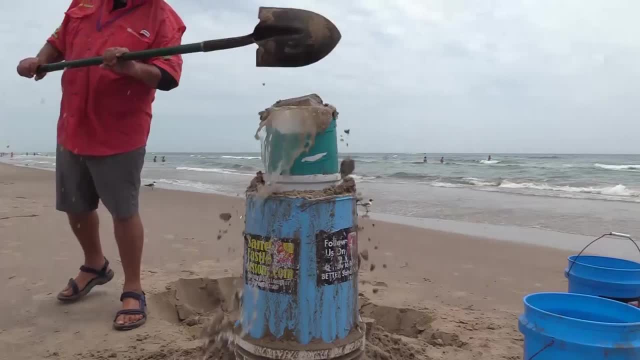 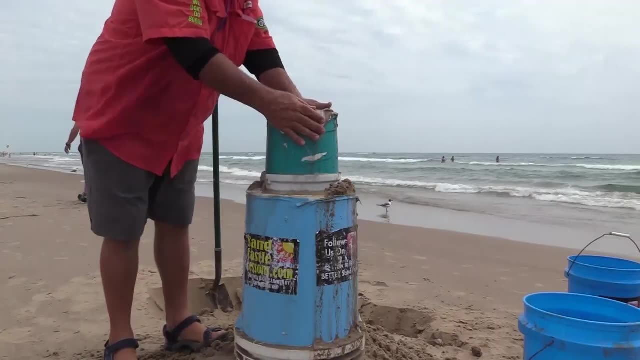 could put our sand through a? uh, literally take the sand, uh, salt, out of it. oh hello, is he doing shoveling, right? okay, guy looks completely mad me, not him anyway. so, uh, we do that and we tap the smaller bucket and uh, and there you go. so we offset it to one side and then 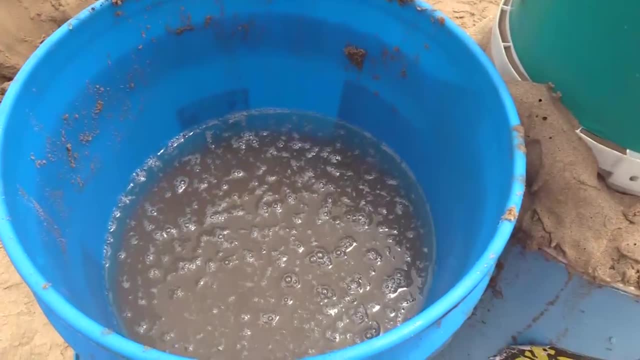 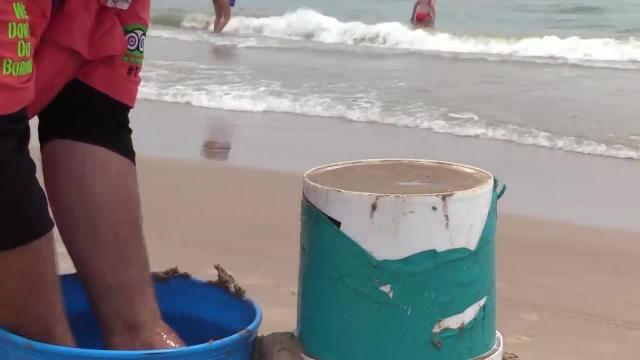 to hand stack. on the top we can hand stack. hand stacking is another technique. there are four techniques in sandcastle building um, and then we put a bit of water on as our bonding surfaces. now we just shimmy. and this is one for the girls. obviously girls, all girls come with shimmying. 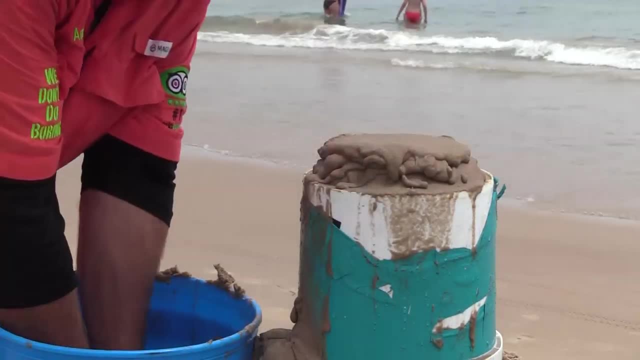 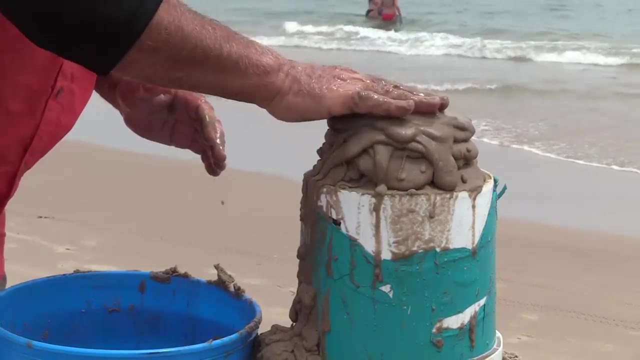 built in. so a girl shimmy and boys jiggle. everybody knows that. so we shimmy and we put our pancakes on the top and they're nice and wet and you can see how fast the water's drying. it's going vroom straight out of the sand, which is great, um, and it means it's uh.